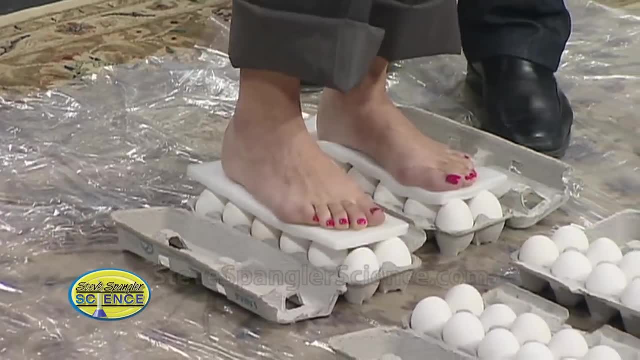 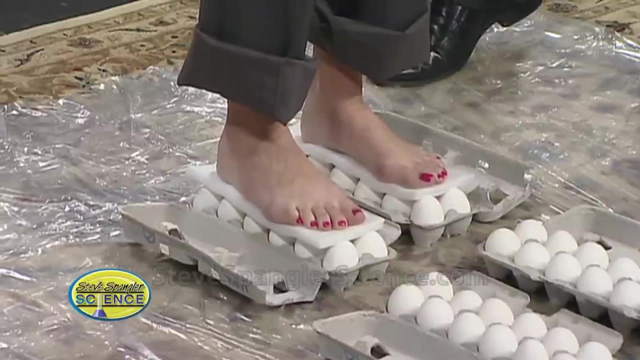 just a little bit. So there's the first one there. Good, Good, Beautiful, You did it. See, you're on a dozen eggs. I'm not holding you, Yeah. So you're on a dozen eggs and everything is just fine, But I think that that's cheating. So 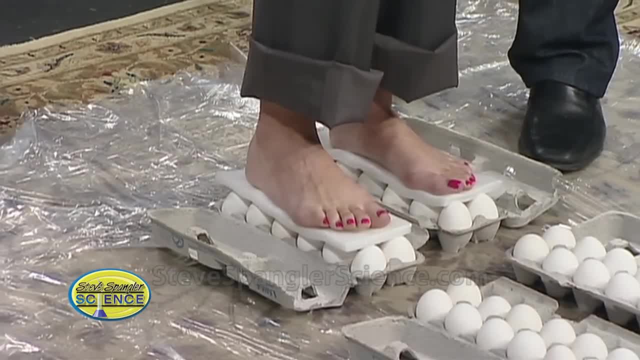 here's what I'd like you to do: Step back, So I didn't tell you about this part. Step back, Okay, Go ahead. Good, Now here, give me your feet and let's take those off. Okay, So here we go, Sorry. 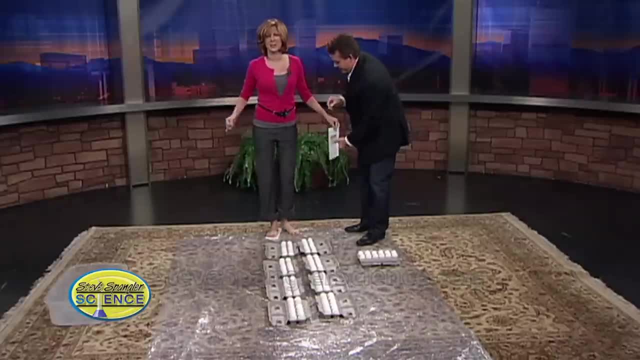 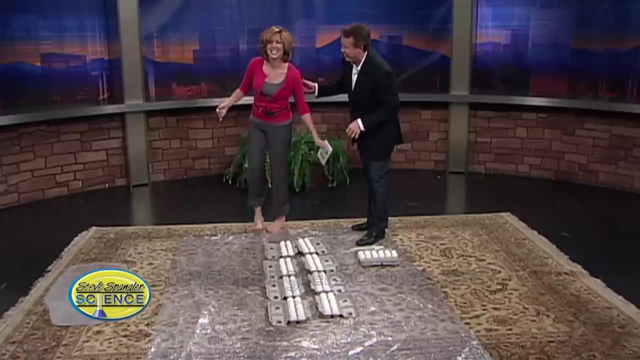 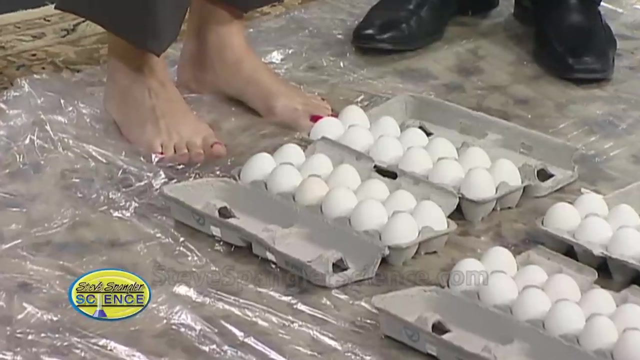 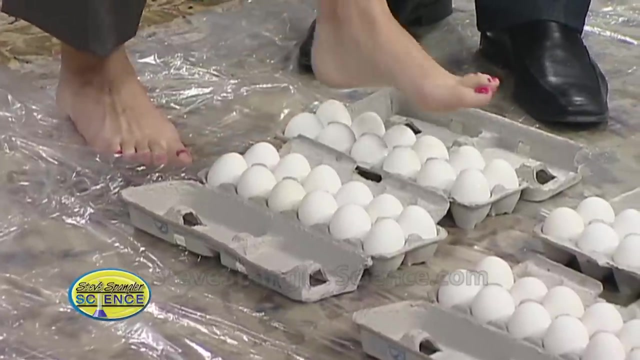 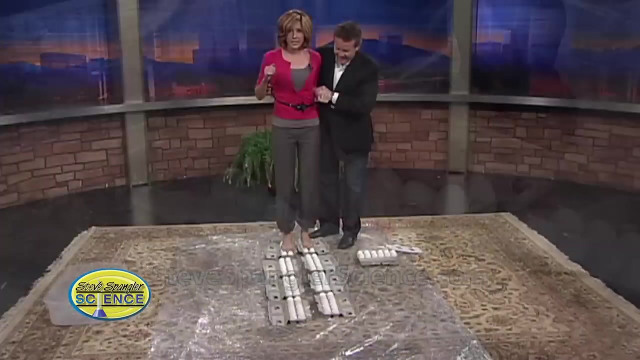 about that. Yeah, Oh, sorry, I know. Definitely duct tape, That's what happened. No, that's gorilla tape, All right, So that's, I didn't want it to come off. Good, And that that small layer of skin that you're pulling off, Yeah, Are you okay? Okay, Good, So now let's do it barefoot. Okay, You just have to be flat footed, Okay. So just just be very flat footed, Okay. So I'm going to help you here. Tell your husband I'm sorry, All right, So here we go. So here we go, Stand in, Good job, Try there, Good, And you're there. Look at this, Okay. Now let's walk Ready. Okay, You can do it, Okay. Okay, Here we go, A little walk. 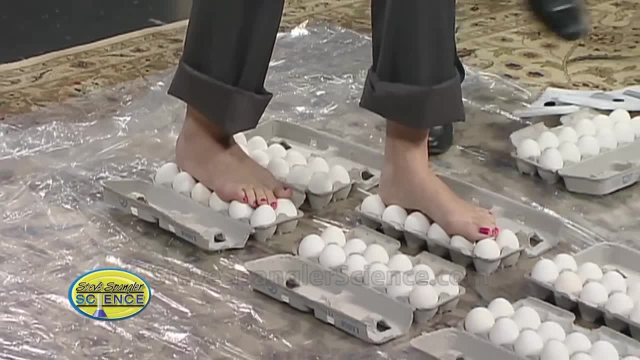 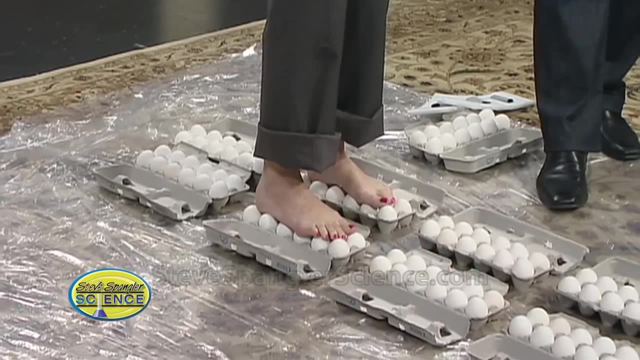 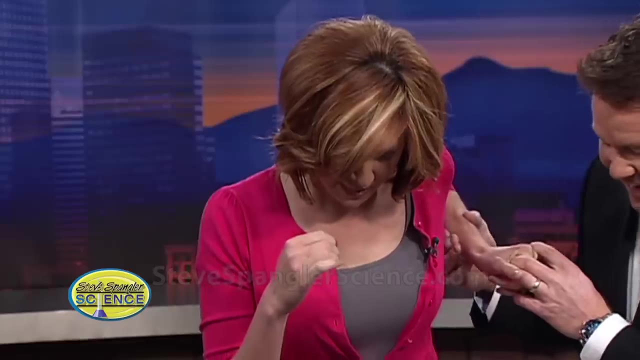 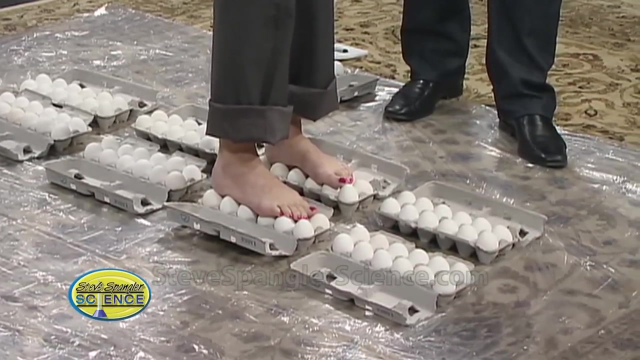 Which foot for? Oh, now, here's the deal is: you're distributing your weight over all of those eggs. So, standing on one egg, bad idea, but standing on a dozen eggs, not bad. And now you're actually standing on 24.. So there you go. That's why the first one's the hardest. Look at this. Is this fantastic? Good, You've gotten through. Let me see You've gotten through. Let me see Six dozen. Okay, Let's do it. Oh, did you just feel one? Oh, there's your foot. It's okay, We're messing around here. Go, go one more. Go one more. There you go, There you go. 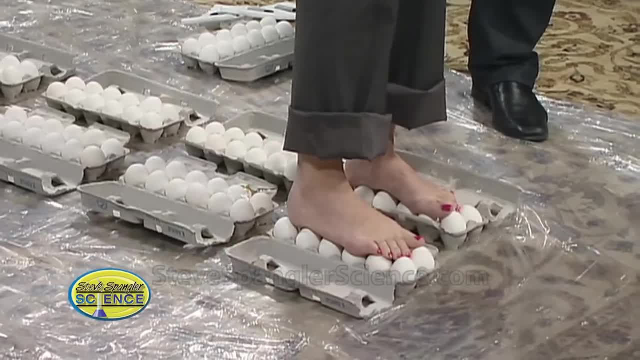 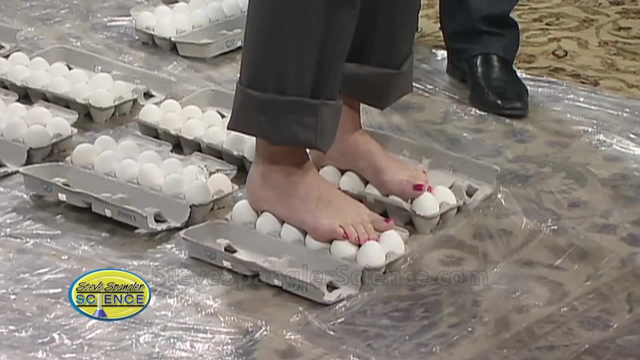 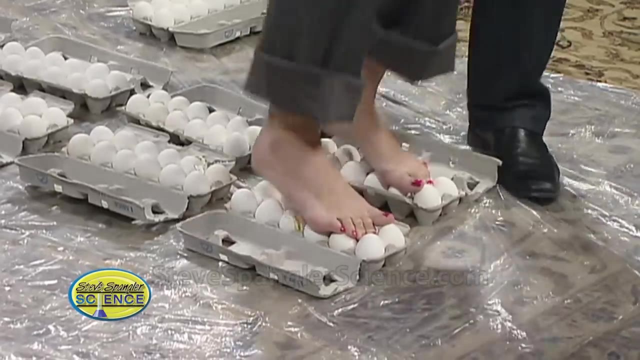 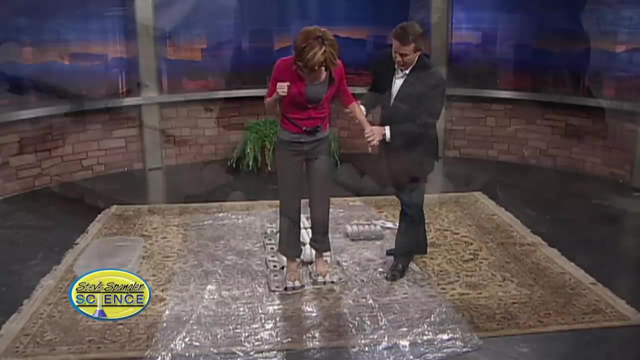 Good job And one more. There you go. Good, Ta-da, She did it And I only broke one egg. You did, She only broke one egg. So there's that one that's broken there. That's perfect. Now watch, If you had more weight on you like this. watch, Definitely, It's amazing. Another one: I'll get how much I put on you. Is that nice? Okay, Give us one jump. Can you give us a jump On to the eggs or off? No, jump onto the eggs. Ready, What? Just jump onto the eggs, I'll help you Ready. One, two, three jump.